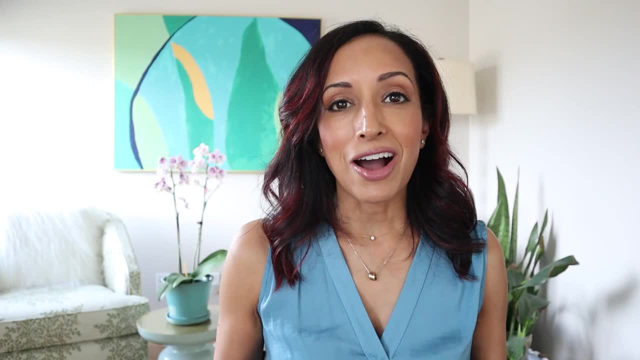 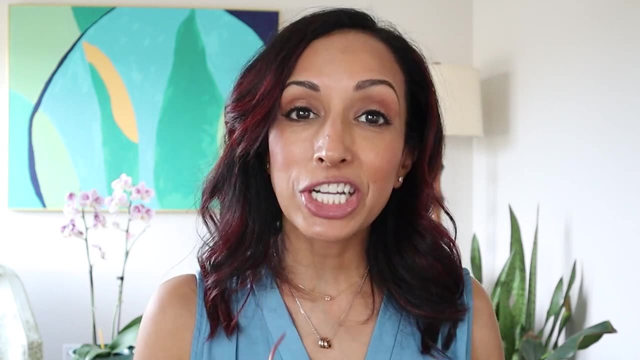 to see that street sign over there. The thing is, it's just not true. Your brain just really likes to have clear vision and you get used to it. The glasses themselves have not changed the way that light is focused on your vision. It's just not true. It's just not true. It's just not true. 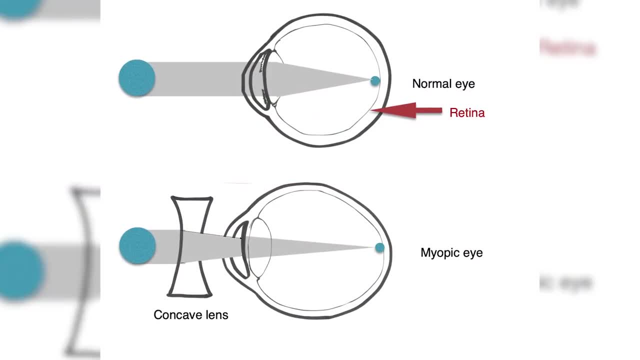 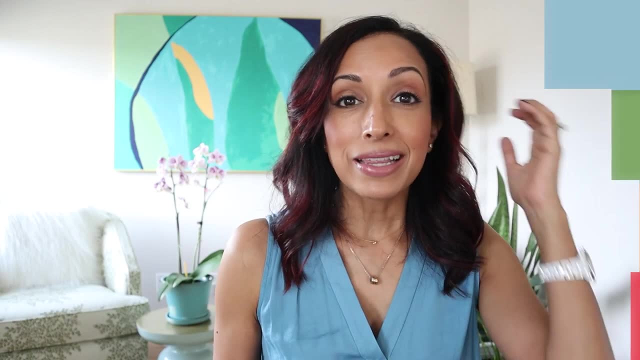 They're not focused in your eye in any kind of permanent fashion. They just haven't. So wearing your glasses absolutely does not create any kind of dependence on them. I know in my mind that it's not true, but it's really easy to fall prey to the fact that it feels like it's so much harder. 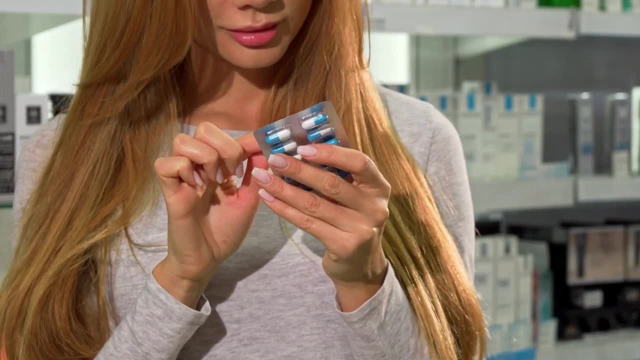 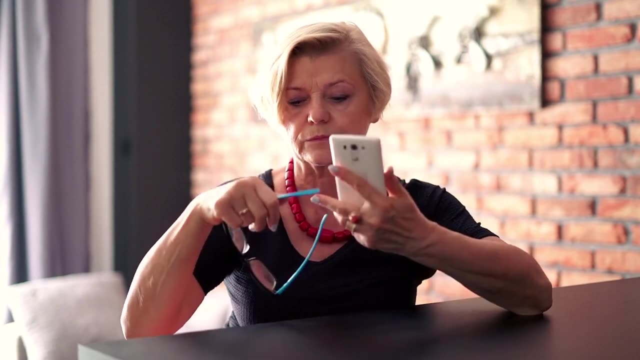 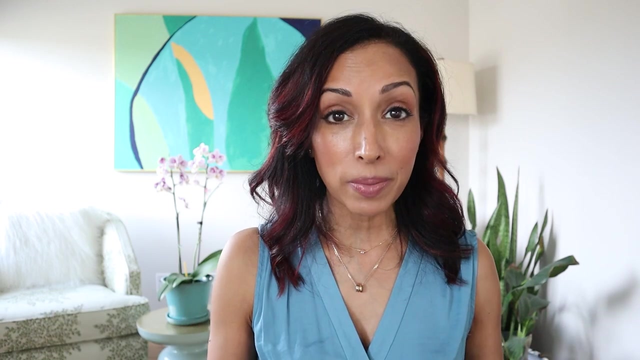 to read a pill bottle, or just even scrolling through my social media. It seems a lot harder now that I'm not wearing my reading glasses, So you've just got to stay firm in the fact that there's absolutely no published data which has demonstrated any kind of permanent change. 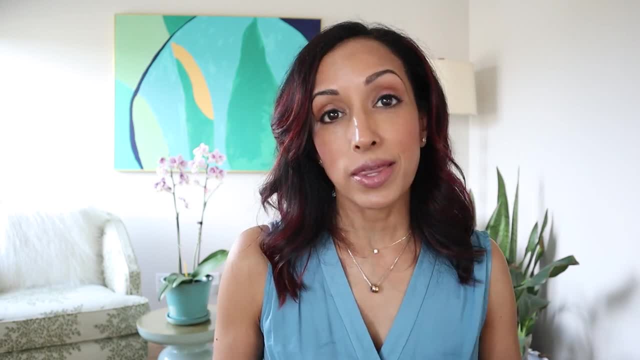 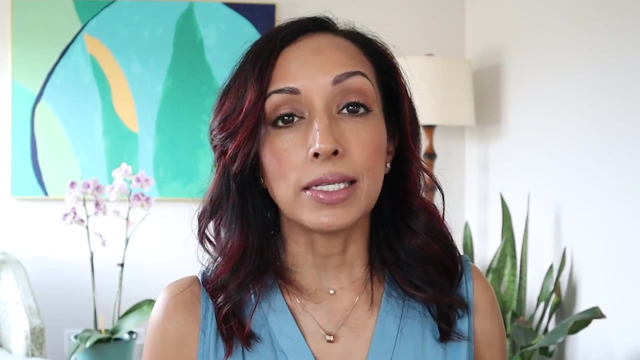 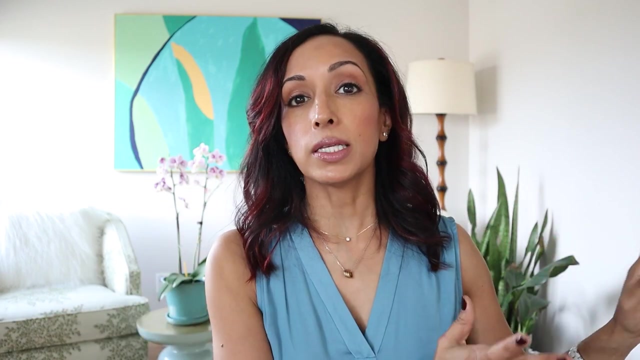 in the eye muscles, the shape of the eye or the way that light is focused. I can tell you that with certainty. Now, what about the converse? Does not wearing your glasses make your eyes weaker? This one's a kind of So for children, it's a completely different situation. Children, younger. 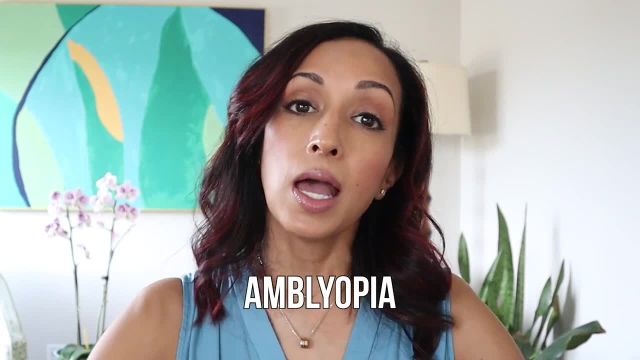 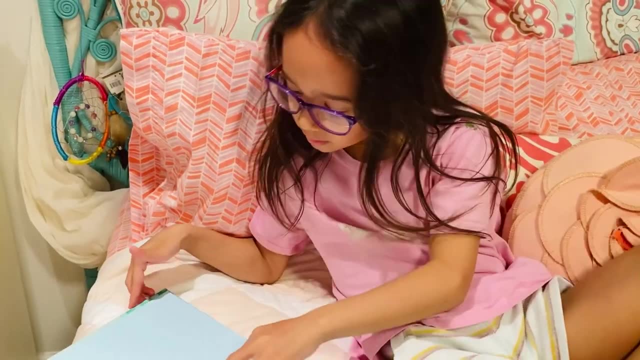 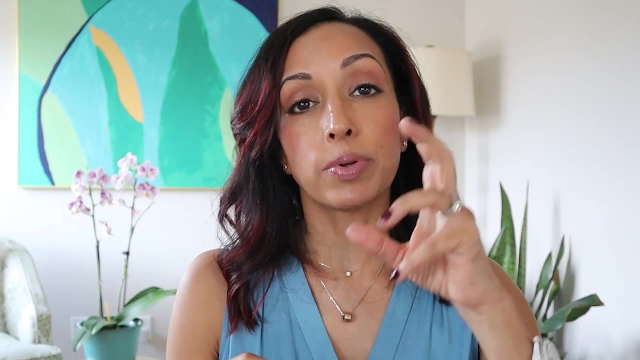 than age 13 can develop something called amblyopia, because they are in the critical period of vision formation. What does that mean? So basically means that when you have a kid, their brain needs clear vision because they are still forming the connections between the back of the eye, between the eye and the occiput, where the vision centers are. So all of 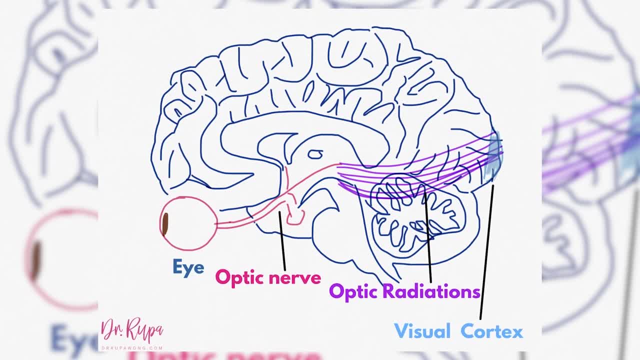 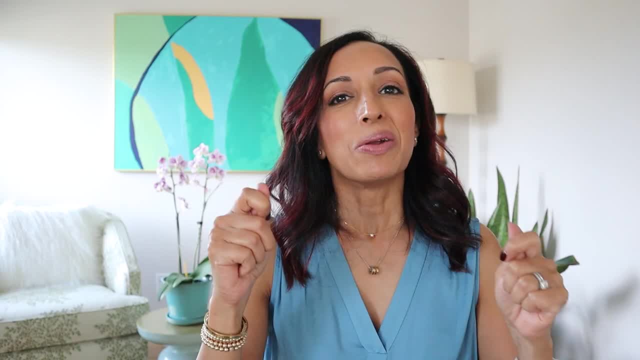 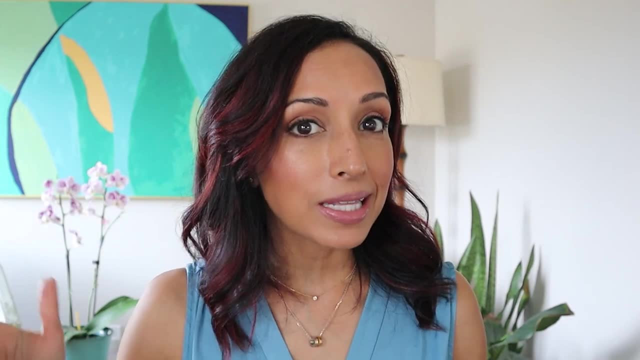 those connections are getting stronger and stronger And they figured this out with these studies with monkeys a long time ago And they actually- it was kind of sad, you know they actually would make the monkeys need glasses. They then basically sacrificed them. 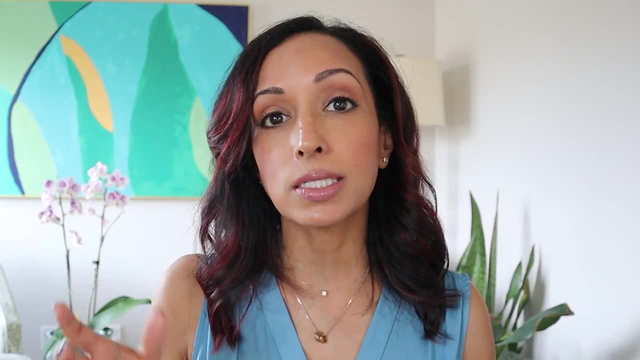 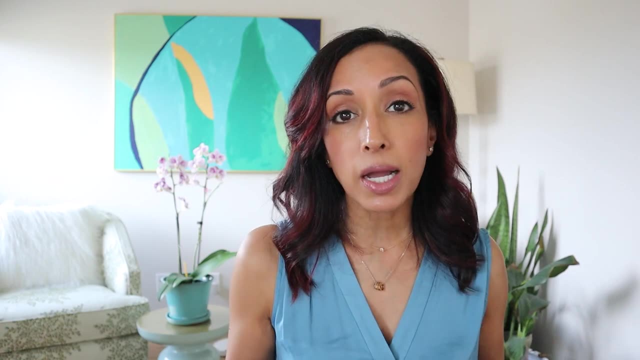 which is the nice way of saying that. they killed them. And then they looked at the brains of them and they saw if it was a very young monkey that needed glasses and they artificially made them need glasses- There's a young monkey that needed glasses and didn't get them. Then those nerve. 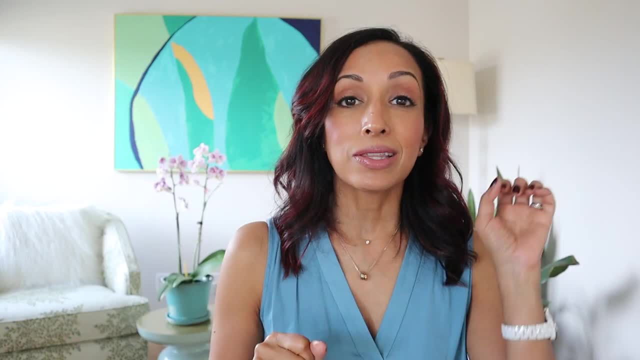 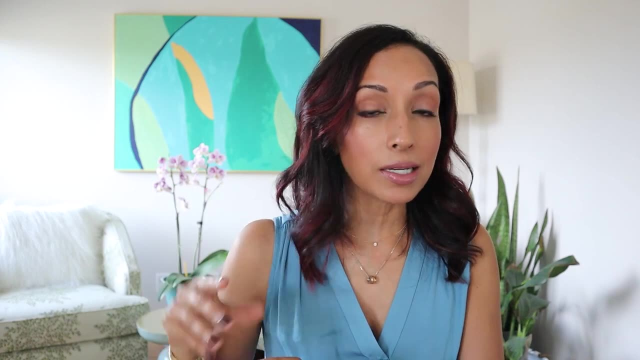 connections look like a tree. So think of it like tree branches, and the side that needed the glasses, that didn't get the glasses, looked like like a little dead tree, versus the side that did not need the glasses was super strong and had lots of sprouts and branches.